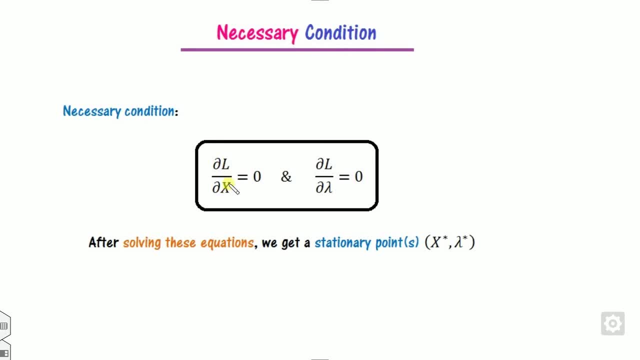 maximum or minimum is partial derivative of x. L with respect to x and lambda must be zero. Once you are solving these two equations, we will get this point. this point is called as the stationary point. After finding the stationary point, we will apply the sufficient condition to 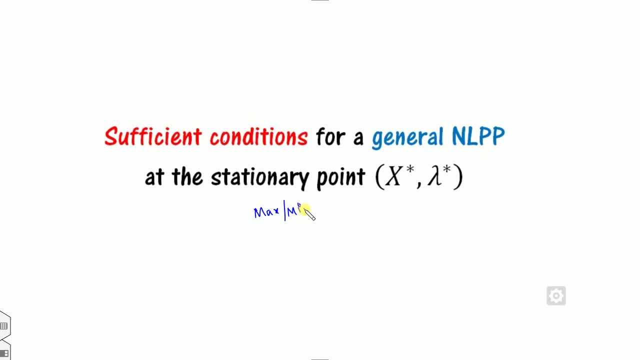 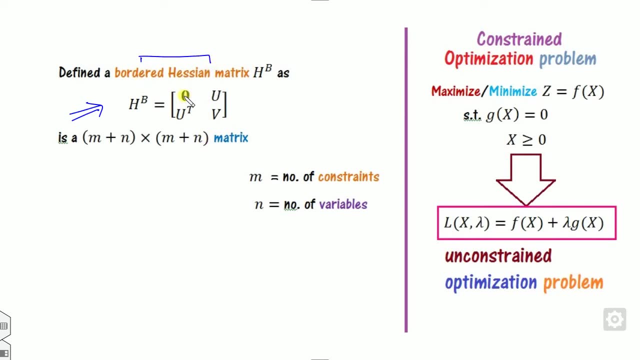 check whether or not it is the stationary point, We will apply the sufficient condition to check the point is maxima or minima. how we can check whether that we will compute this matrix that is called as the border Hessian matrix and this is form of zero: u, u transpose, and v the size of this. 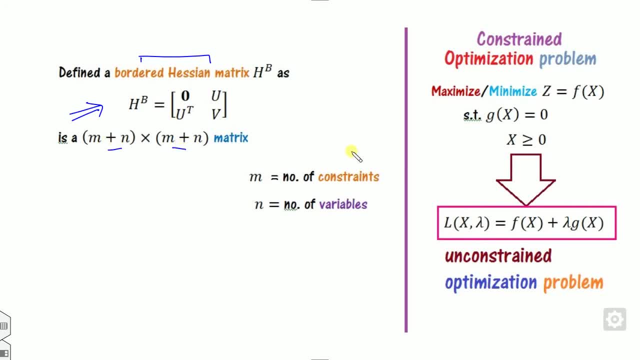 matrix is m plus n. m plus n. what is the? m is number of the constraints, like, like. say this: how many constraints are there? n is my number of the decision variables. how you find the u, u is nothing but my partial derivative of this. constraints with respect to the x and v is nothing. 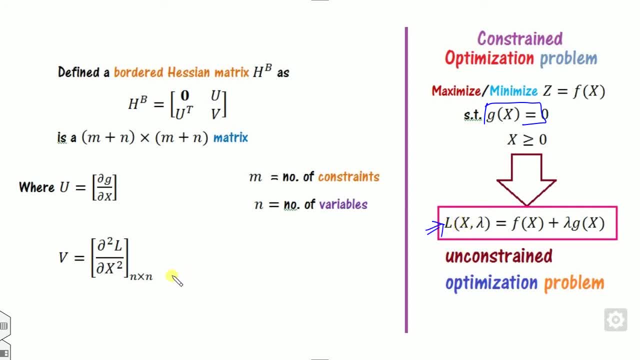 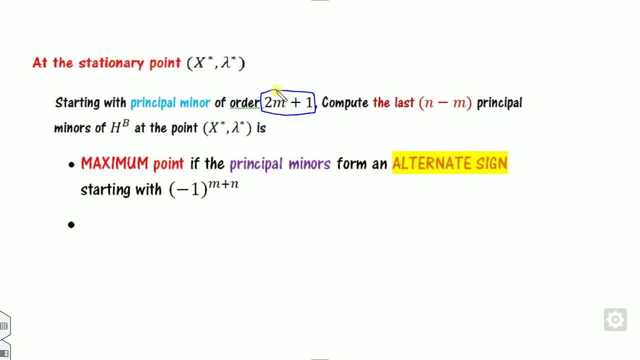 but my partial second order, partial derivative of this L with respect to x. once we will construct this matrix, then now it has m plus n cross, m plus n size. so we have to find the principal minors. remember there are the two conditions. one is only 2 m plus 1 and this is n minus m, this n minus m. 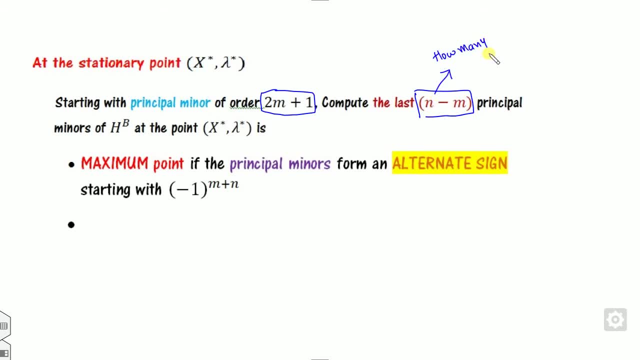 conditions will tell us how many minors we will calculate. this is tell us how many minors we will calculate, but since this, the size is m plus n, cross m plus n, and this 2 m plus 1 will tell us from where, tell us from where we can start, from where we can start. so remember that. so this 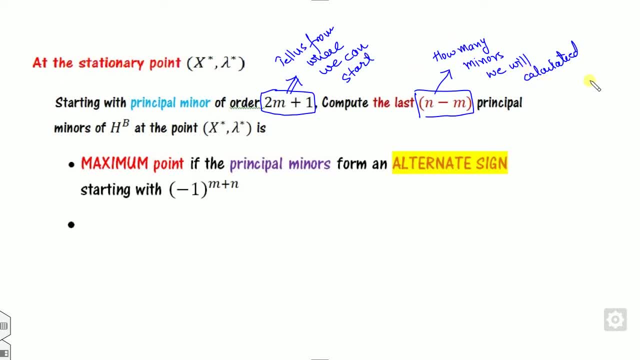 n minus m will tell us how many minus will be calculated, and 2 m plus 1 will tell us that from where we can start. once we will come compute all the principal minus at this point, then we will check whether they are of the alternating signs. provided the first sign will be of this nature, then it's. 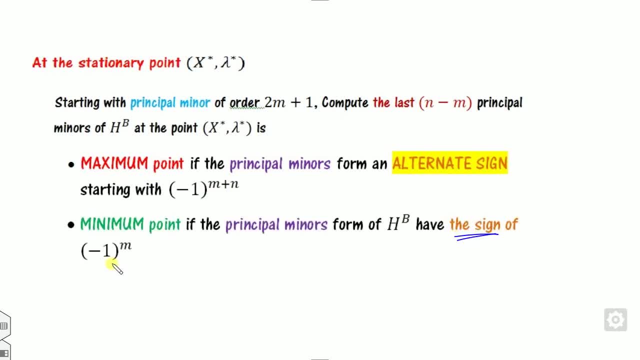 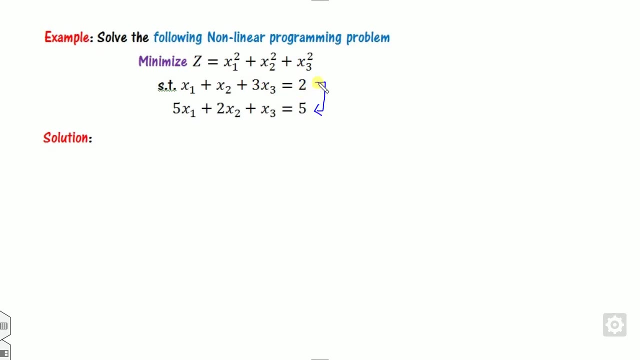 the maximum. and if they are same sign as that of this, remember, if they are alternative, then it's maximum. if they have the same sign, then it's a minimum. starting from this or this, let's discuss some examples. we will follow the same rule. look at that. how many constants are there? there are the. 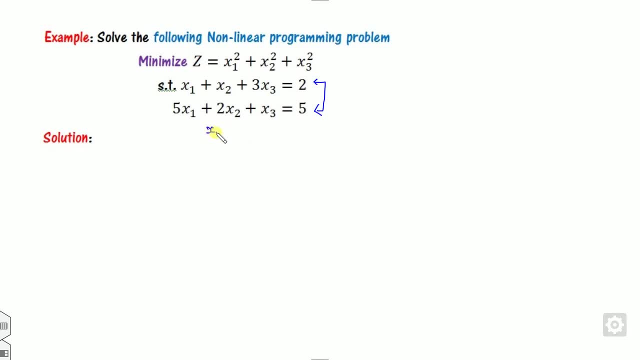 two constants and look at that. what is the nature of the x1, x2, x3? it is clearly sees that they are my, because x1- x2 is not greater than 0.. so first thing is we have to define the lagrangian function. 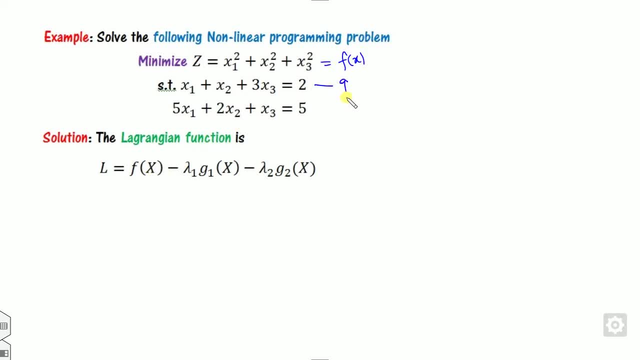 that is f of x. this is my fx. the first constant, g1. second constant: g2. so after substitute, the value of here, this is the fx. g is now right hand side must be 0, so i can take 2 on the left hand side. this is the third second constant. once you are defining this l, now we can define the. 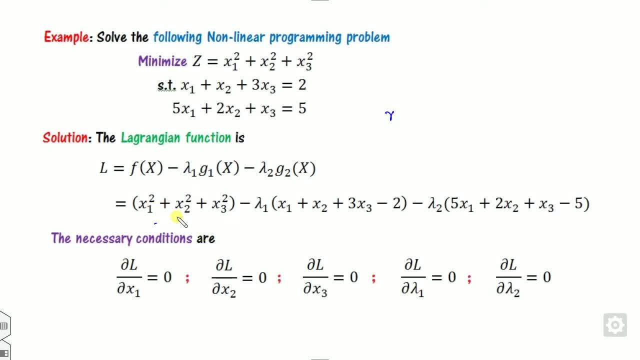 necessary condition. how many variables are there? one is the x1, x2, x3, lambda 1 and 2. all must be 0. for example, if you take the partial derivative of this with respect to x1, it gives 2, 2, x1 minus lambda 1, minus of 5. lambda 2 is 0, similarly for the second, and so on. 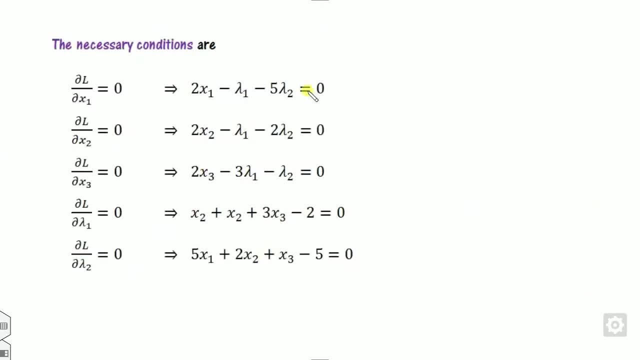 once we will compute all we get here now. remember that we will follow the same method which i discussed here for all the other problem as well as the remaining ones. so from the first one we will find the value of the x1, from the second we will find the value of x2. 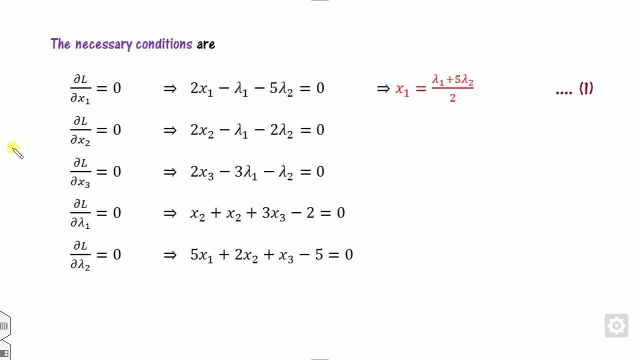 from third we will find the value of x3, and so on. So look at that: from here we can find the value of x1, from second we can find the value of x2,, from third we can find the value of x3.. Now, after 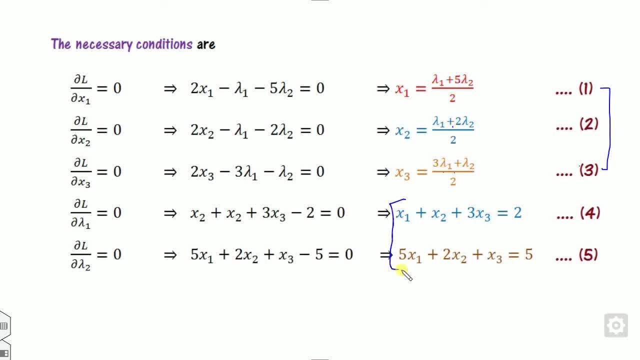 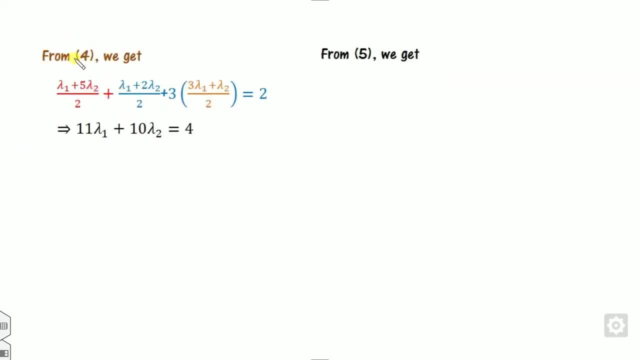 substitute this value of x1, x2, x3 in these two equations, 4 and 5, the resultant equation will be in terms of lambda 1 and lambda 2. like this way We can substitute the value in 4. after simplify, we will get this equation. Similarly, after substitute in equation number 5, we will get: 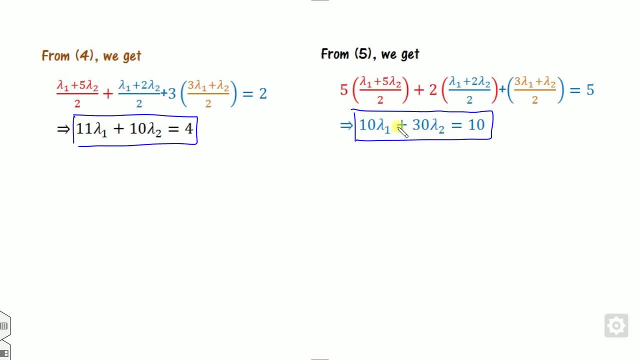 here Now. these two equations are lambda 1 and lambda 2. you can simply solve with the help of the calculator. You can simply solve it with the help of calculator. you will get these two equations. Once you will get the lambda 1, lambda 2, we can substitute the value of this in x1,, x2, x3. 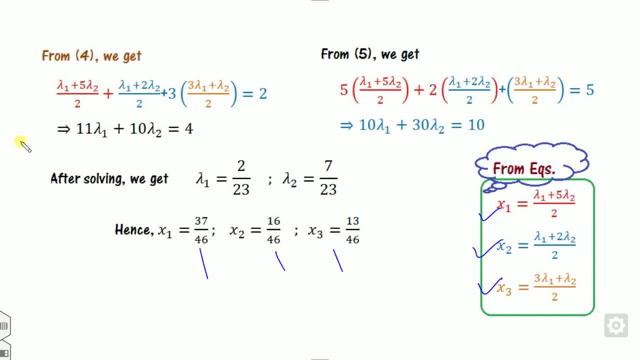 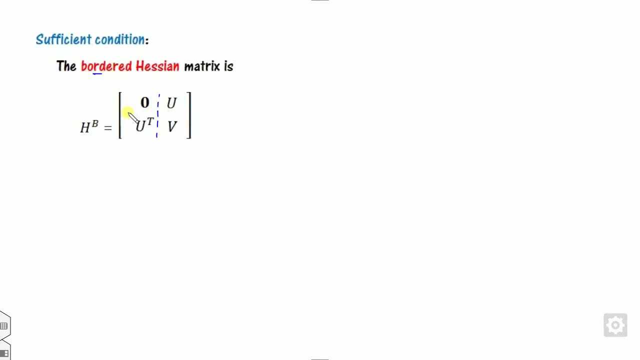 we will get these three points. Hence the stationary point will be x1, x2, x3, lambda 1 and 2.. To check whether this point is a maximum or minimum, what we will do, we will apply the sufficient condition. We will check the border, Hessian matrix, that is u v and there First of. 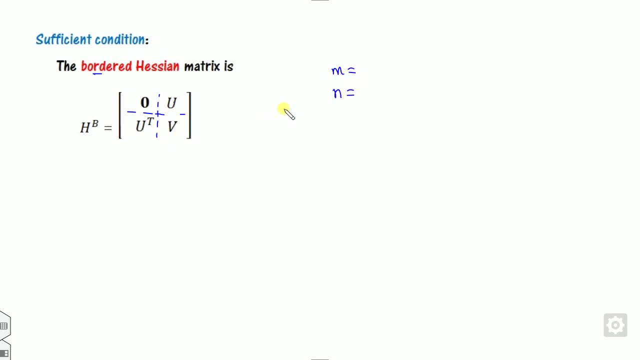 all. what is the size of this? we will check. what is the m? what is the n? m is my number of the constants. Look at that. this is my original problem. How many constants are there? 2. How many variables are there? 3. So it will be my 5 cross, 5 m plus n, m plus n. Now what is the value? 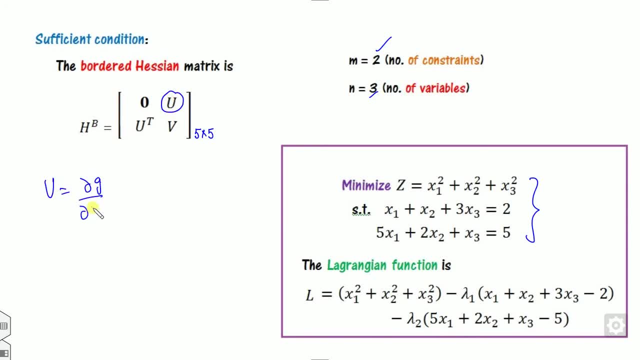 of u? All of you know that. what is the u? m plus n? m plus n? Now what is the value of u? m plus n? m plus n? m plus n? So what is the u? m plus n? m plus n? Now what is the u? m plus n? m plus n? So 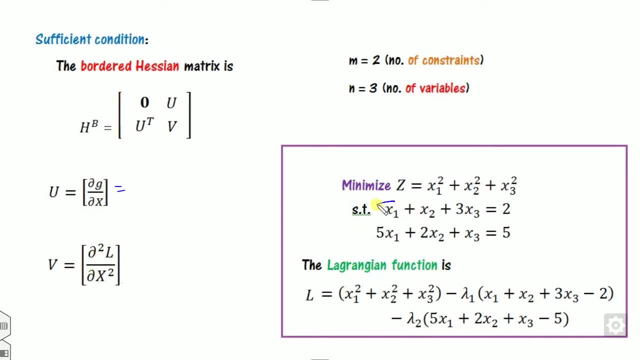 you can see that. So what is the part? This is my g. Now the size is 2, so it will be my 2 cross matrix. So what is the first derivative with respect to x size? First one is with respect to x1, then x2, then x3.. Similarly, for here, this is my u 1, that is partial derivative of g with. 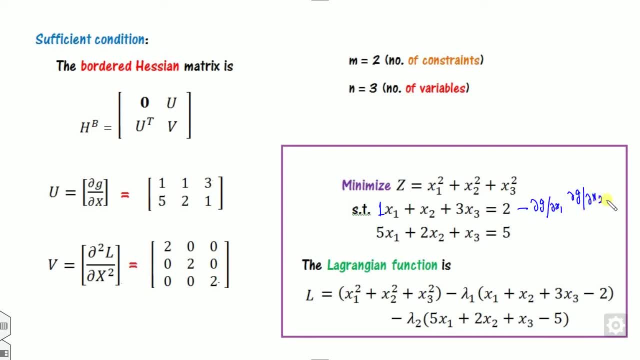 respect to x1, partial derivative of g1 with respect to x2, and so on. Similarly, for here, and what is the v is partial. second order: partial derivative. this means partial derivative with respect to x1 square. this means partial derivative with respect to x1, x2. this means: 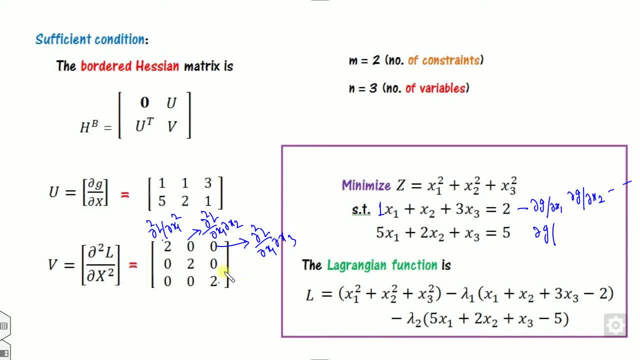 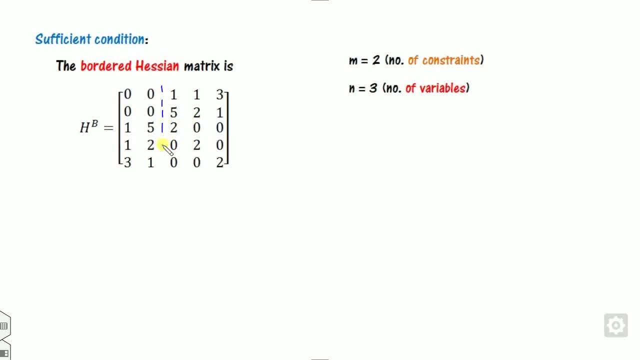 partial derivative with respect to x1, x3 and so on. so once we will calculate u and v- now look at, this is a transpose- we can substitute this value in here. so look at that. this 0 is my nothing but a 2 cross 2 here. now the size is my 5 cross 5. so now our task is to calculate the principal minus. 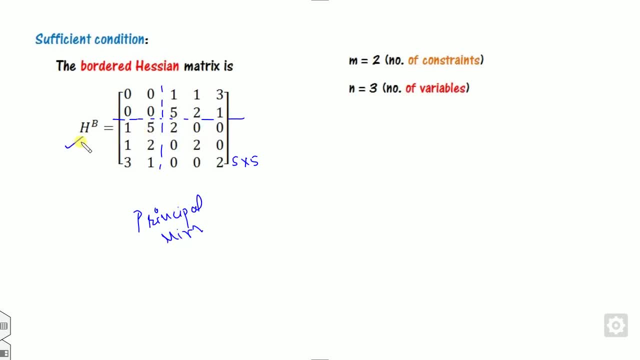 how many principal minus we will calculate for this hb. that will tell us about the n minus m. so what is the n value? of the n minus 1 is 1. it means we compute only the one principal minor. what is the order of the first principal minor is? is it d1, d2, d3, 4 and 5? that will tell us from the. 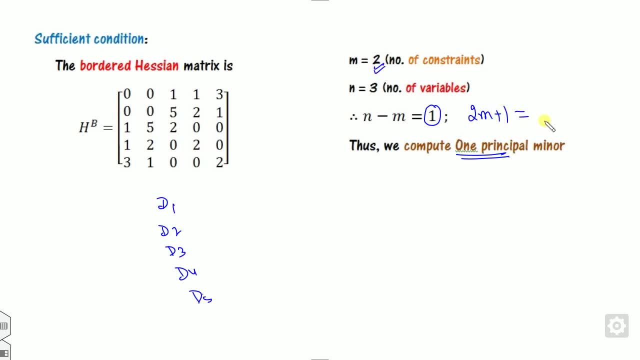 2m plus 1. what is that? 2m plus 1 is m. 2m plus 1 is m. 2m plus 1 is m 2, it is 5. so therefore we will calculate the one principal minor whose size is 5. what is the? 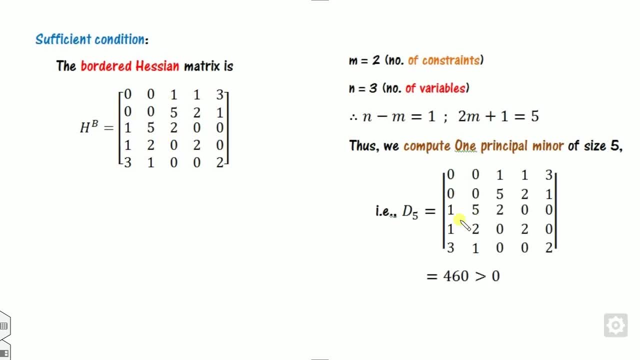 principal minor, whose size is 5. that is itself we will calculate, and it comes to be 460. now check what is the sign of this. is it of here? then it will be of maximum. if it is of minus 1 raised power m, then it will be of minimum. so what is the m? is my 2, so what is that? this will be my 5 and it's a. 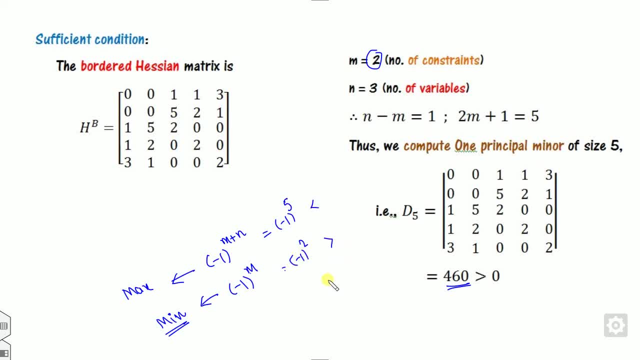 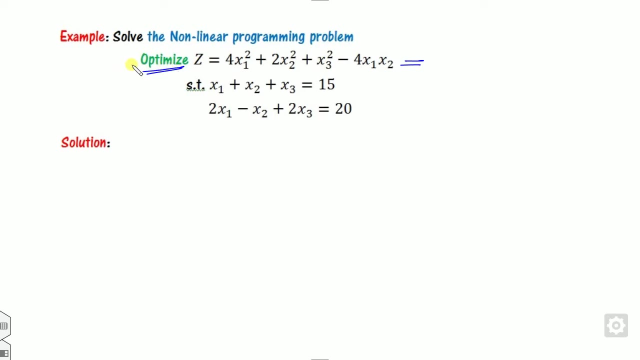 negative and but it is a positive. so since this is accordance with the sign of here, so therefore by the sufficient condition, it will give a minimum. now we will apply the same method for this second example. again, you can see now look at that. this is optimized either. it can be maximum. 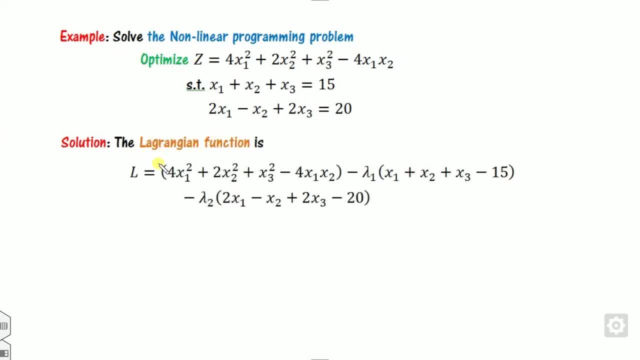 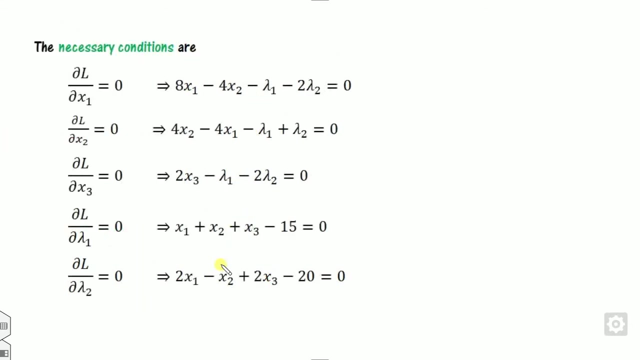 or minimum. we will see what will happen. we can define the l by using the 2l. lambda 1 you can take as a plus as you wish, because if it is a unrestricted variable, again there are the five unknown parameters. we will take the necessary conditions as here, again from the first equation. 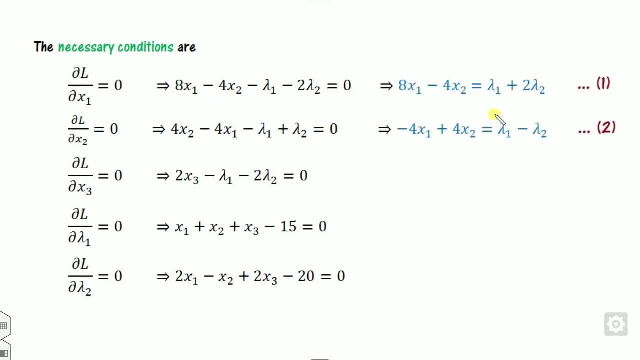 we will take the value of x1 and x2, like this here from third, you can easily find the value of x2, like this and so on, how you find the value of x1, x2 and so on. so you can simply see if you can. 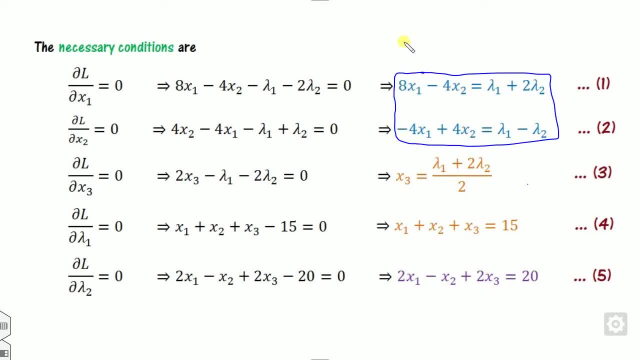 from the first and two, can you? if you simply add, what will happen? this is nothing but my here. so from the equation this you can take the value of x1. similarly, you can substitute the value of x1 in either of equation. you will get the value of x2. 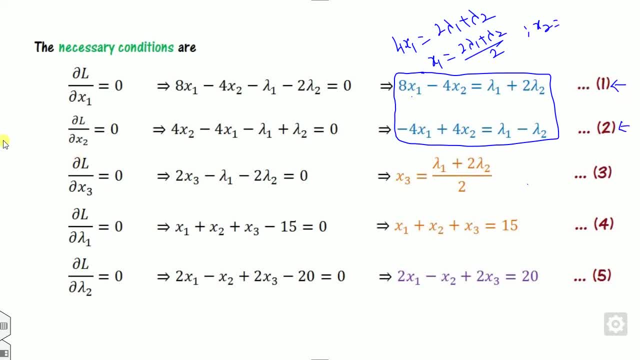 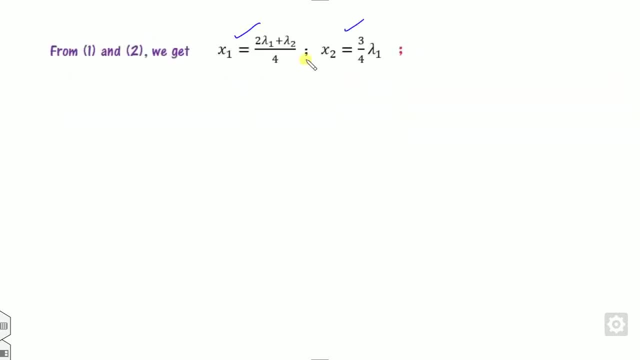 it means by by solving 1 and 2, you can get the value of x1 and x2 already. we have known the value of the x3, so x1 and x2 we already calculated, x3 we already known, so we can substitute the value. 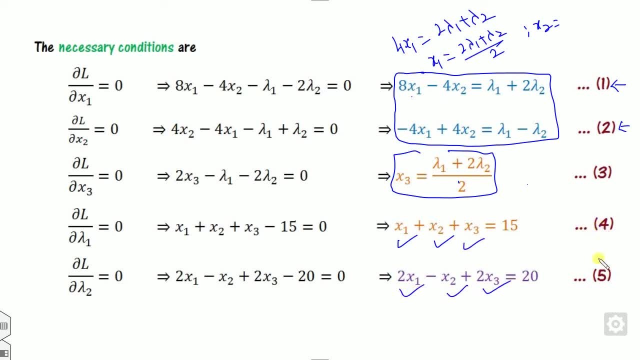 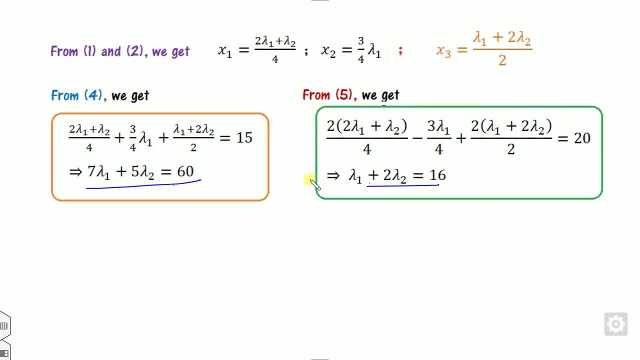 of x1, x2, x3 in these two equations, that is, 4 and 5. after substituting these two equations, we will get these results out there. now you can simplify these two equations with the help of the calculator. you will get the value of lambda 1 and lambda 2. 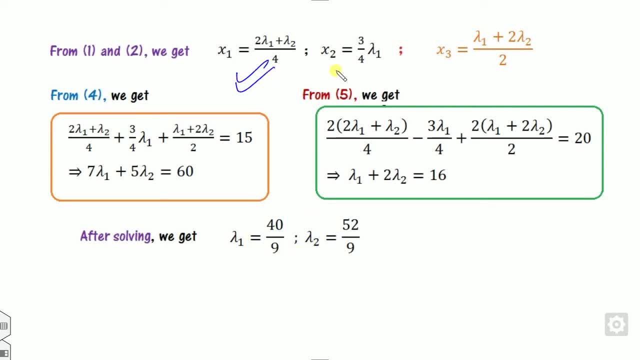 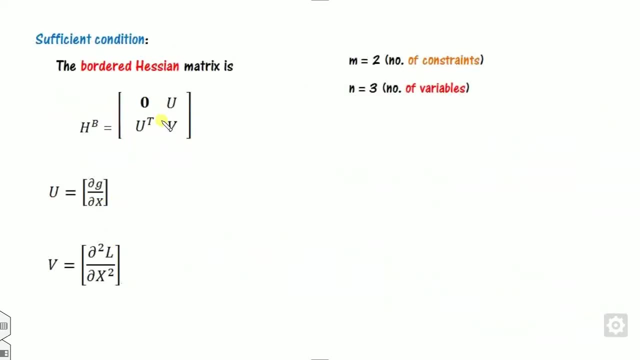 here, after finding these two values, we can substitute the value. here you will get the value of x1, x2 and x3. therefore the stationary point is here. to check whether this point is maximum or minimum, we have to calculate the hessian matrix like this way. in this again, case m is my 2. 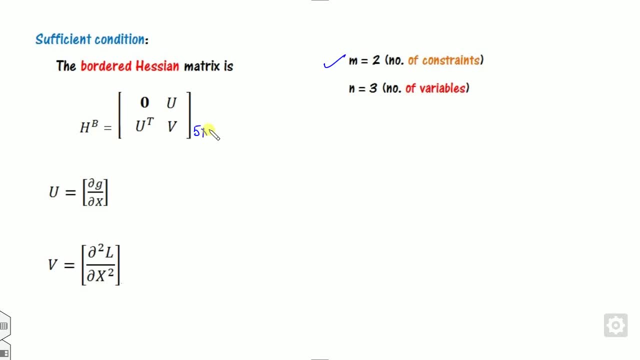 n is my 3, so it will be again 5 cross 5. what is the value of the u is? look at that. this is the matrix. so what is the partial derivative of? this is 1, again his 1. this is 1, this is 2 minus 1, and so on. so remember that if, for example, if my problem is like this way: 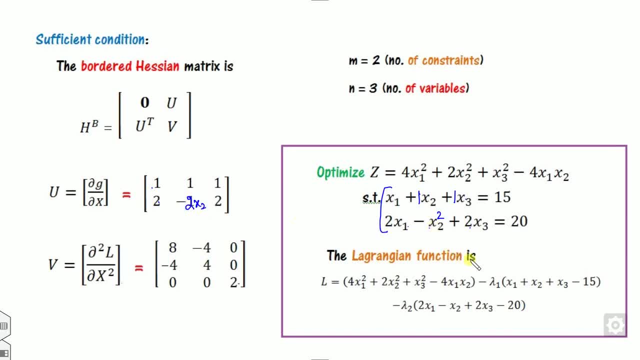 so then it will be my 2x2 and so on. so, similarly, from here you can find the value of v as this: once after finding this value, you can substitute the value here. you can see here. so if in now we have to find the value at x1, 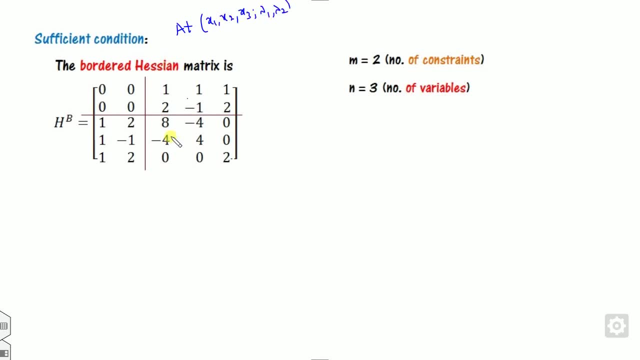 x2, x3, lambda 1 and lambda 2. if any of the values appear here, we can substitute the value correspondingly here. so now it is a 5 cross 5, so we will check how many principal minus we will compute. that will tell us about n minus m. so we will compute only one principal minus, what is? 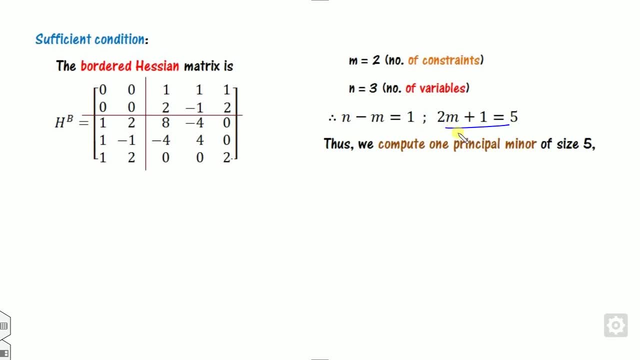 the size of this principal minor. that will tell us about that: 2m plus 1, so that is a 5. so we will compute the 5 cross 5 matrix. that is a itself matrix system. so now it will be of the positive sign. so if 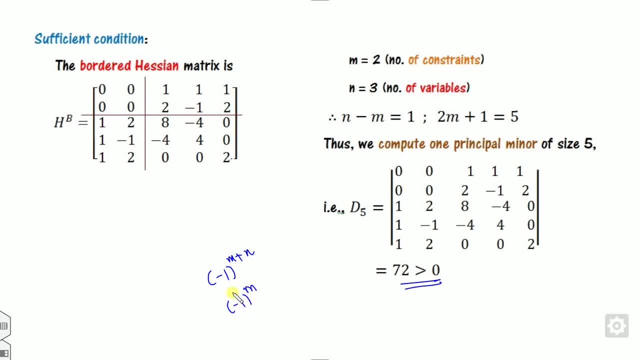 check whether this is a sign of: according to this or according to this, it will happen for the maximum. it will happen for the minimum. so, since this is the sign corresponding to this, because m is my 2, so it will be positive. what is the m plus n is 5, so it will be negative. so 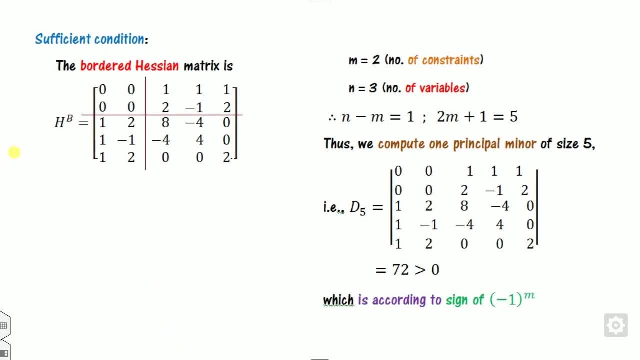 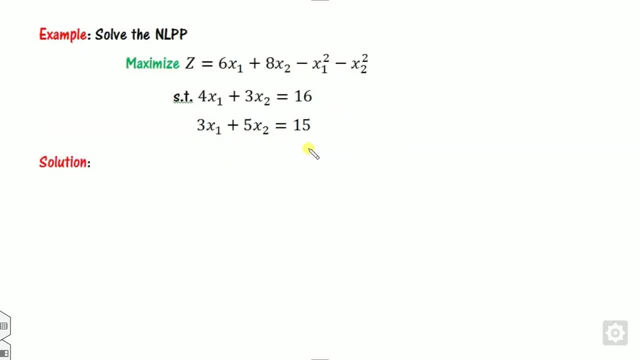 therefore, this stationary point is my minimum. look at one more example. we will again apply the same rule. again, there are the unrestricted, whatever is there. so we will define the l value. how many decision variables are there now, in this case, x1, x2, lambda 1 and lambda 2. there are, the 4 are. 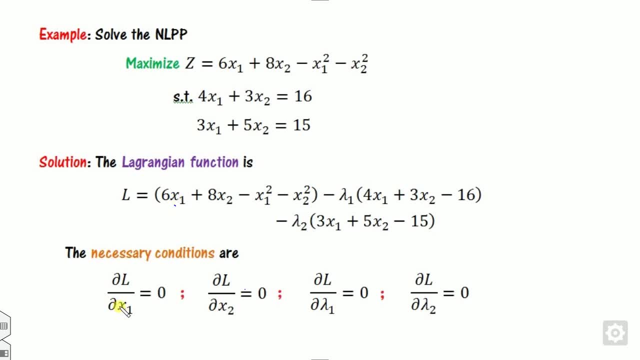 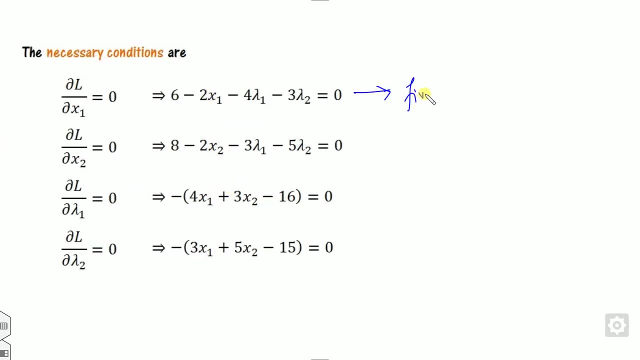 there. so after derivative this we can see what is. the derivative with respect to x1 is 6 minus 2x1 minus 4. lambda 1 minus 3 is 0. this is with respect to here. similarly, for the others we can compute. here again, we will follow the same rule. from the first we can find the value of the x1 second from 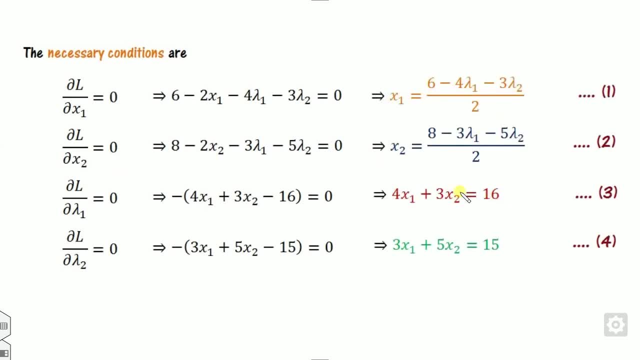 the find of the x2. we will get these four equations. so look at that. we can substitute the value of the x1- x2 in these two equations. else we can simplify these two equations and we can find the value of the x1 easily. we can find the value of x2. 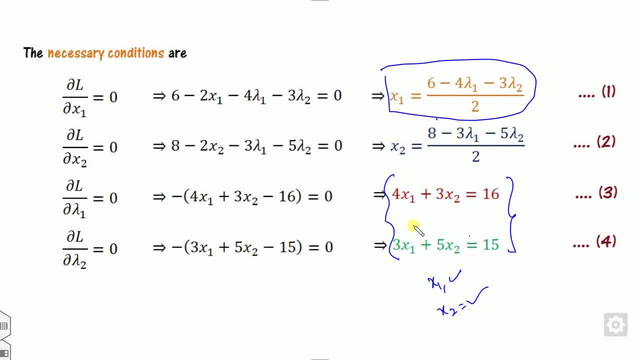 after finding the value of x1 and x2 from the third and fourth, we can substitute the value here. this will give you the value of the lambda 1 and lambda 2. that's depending upon you, but i follow the same rule as we discussed in the last example. from the equation 1 we can find the x1, x2 we can. 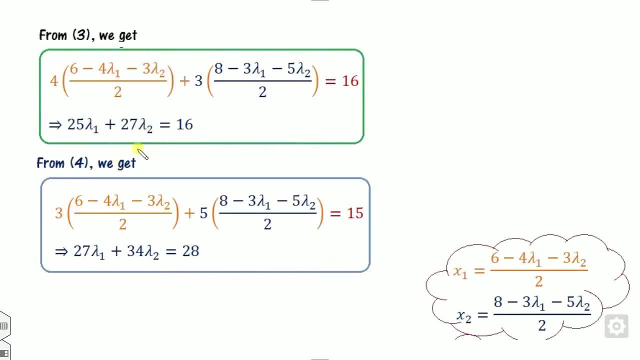 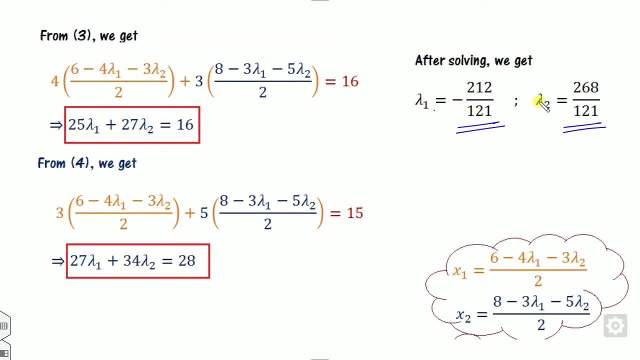 substitute both the values in third and fourth. we can get. these values are there. we can substitute these two values, x1 and x2, in here. now look at that. this is the value of the lambda 1 and lambda 2. after simplify, we can get the value of this. once you know the lambda 1, lambda 2, you can. 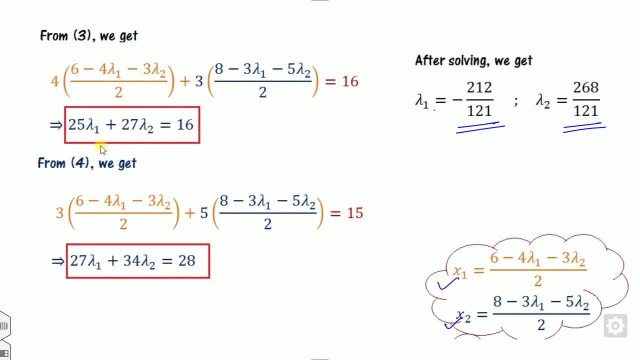 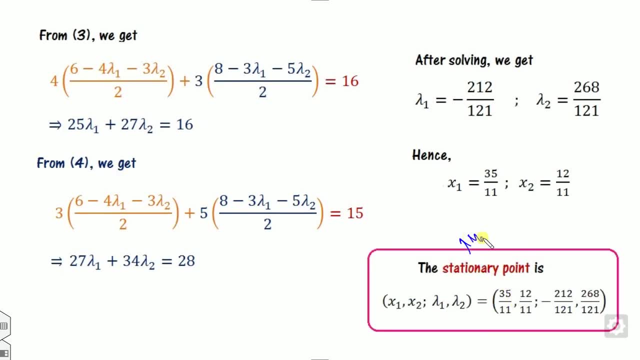 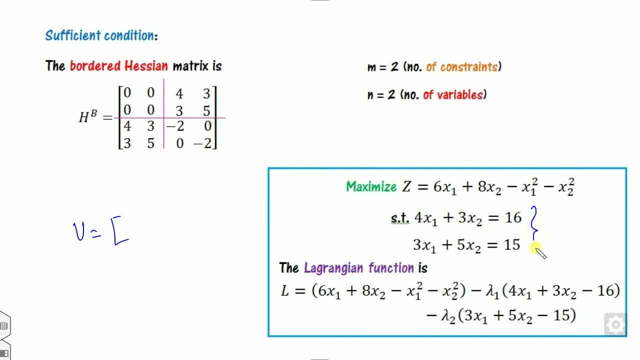 substitute the value of the calculated x1 and x2, you can get this point. therefore, your stationary point will be here again. to check whether this point is the maximum or minimum, we have to again draw the border. hessian matrix. look at that. what is my u is the derivative of the g constant. that 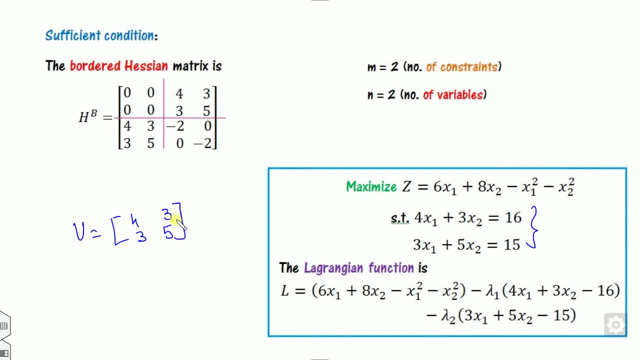 is a 4, 3, 3, 5. look at that. this is my u and this is the u. transpose what is the v is partial derivative. now it's a 2 cross 2 because there are the two variables. so it will be x1 square partial. 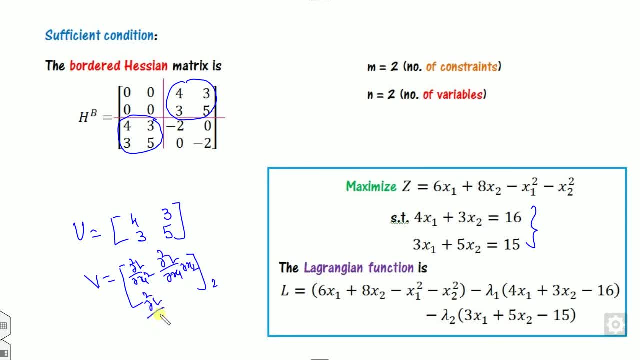 derivative with respect to x1- x2. this is l of x2- x1 and this will be x2 square. so what is the positive of that? that will get this value? we will get the minus of 2. this will be the 0, 0 and minus of 2 here. now it will be my m plus and there is a 4 cross 4. so how many principles minor?